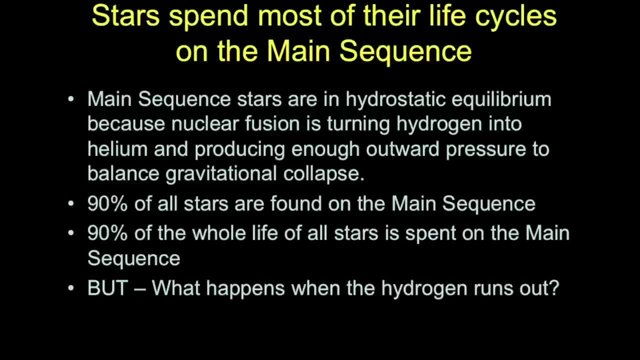 observe, are going to be in this stage of their lifetime, all of this time turning their core hydrogen into helium. That's the fuel that they use to sustain their energy generation and this balance between gas and helium. But when the hydrogen fuel in the core runs out, that's when a star is no longer a main. 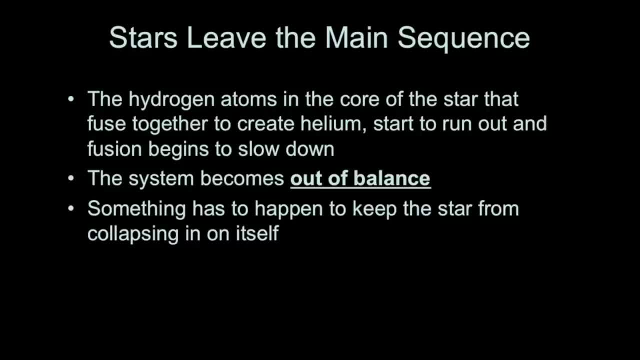 sequence star, and it becomes something else. When a star leaves the main sequence, that is, when it finishes using up its hydrogen fuel for nuclear reactions, it becomes out of balance. There is no longer a sustained set of energy-generating processes in the 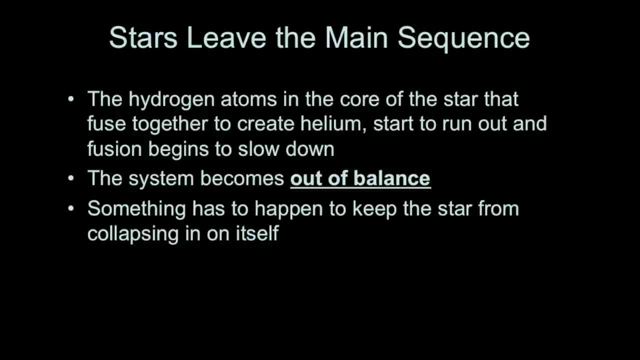 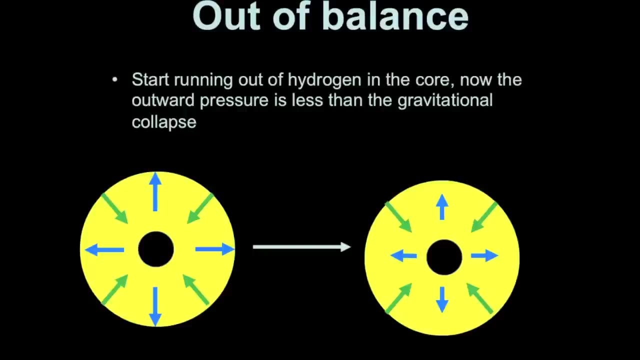 core to counteract the crushing force of gravity on the inside of a star, and so the competing pressures are no longer in balance, and eventually something has to keep a star from collapsing in on itself. So what's happening on the inside of a star When the hydrogen is completely converted? 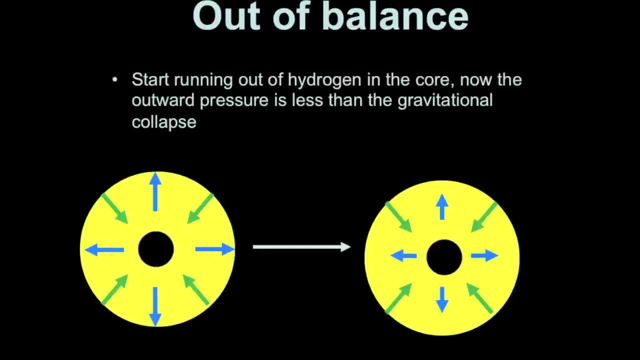 into helium in the core, then you've got less gas pressure pushing out, and that's demonstrated, or at least depicted in this diagram, where we have a balance between forces on the left- that's the main sequence star- where gas pressure, which is the arrows pointing outward, is balanced. 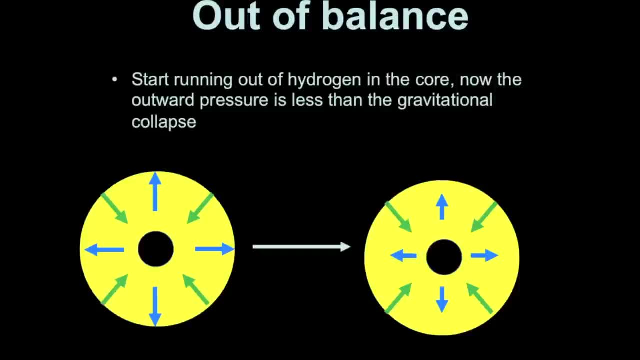 with gravitational pressure, the arrows pointing inward, And then, on the right side, we've got the follow-up situation. When the hydrogen fuel has been used up now, the core will have less sustained energy generation and eventually no more. So what's happening on the inside of a star? When the hydrogen fuel has been used up now, the core will have less sustained energy generation and eventually, 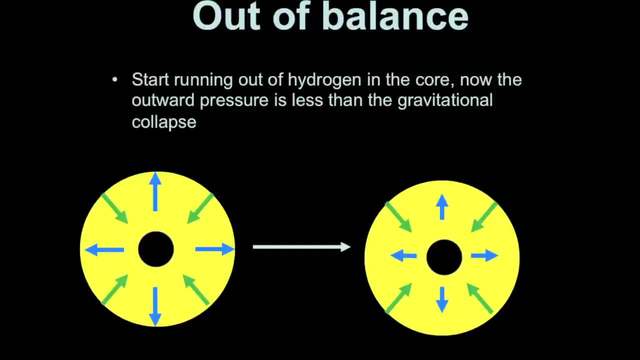 none, And so the arrows pushing outward will not have as much pressure compared to the inward gravitational pressure, and so there won't be a balance and the net pressure will be inward. The star will effectively get smaller. it will begin to collapse. 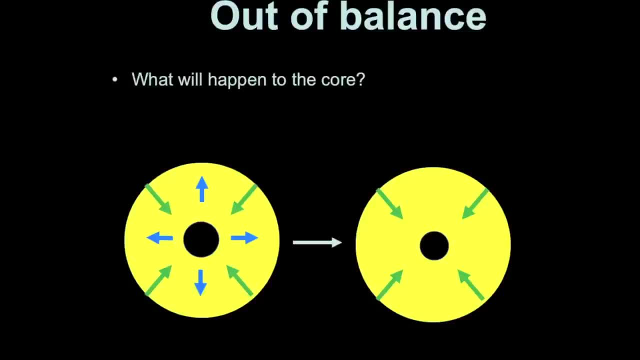 So what happens to the core? Well, we have to differentiate between the outer layers and the core of the star. The core itself will be completely helium. That helium is not fusing into any new elements at this point, but it's still extremely hot. Gravity is. 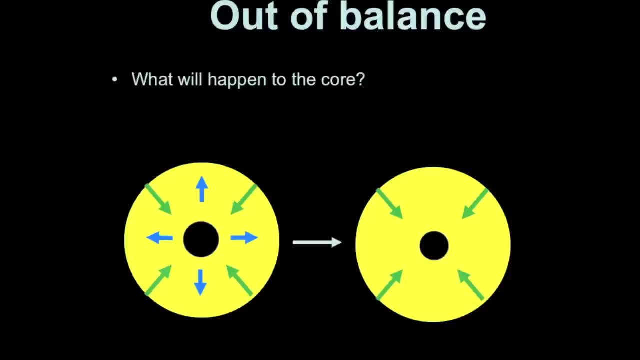 going to crush the helium atoms into an even smaller size and as that occurs, the helium core will get hotter, denser and will eventually begin fusing, but not yet. The outer layers will also collapse down onto the core. The outer layers of the star are just hydrogen. 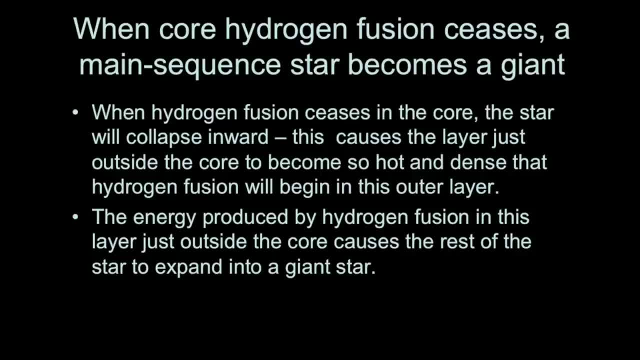 atoms which have not, to this point, been fusing. While the core is collapsing into a very dense, hot ball of helium, the outer layers are compressing a very dense layer or shell just around the core. This is just hydrogen atoms, but they get so hot and so dense in that shell around the 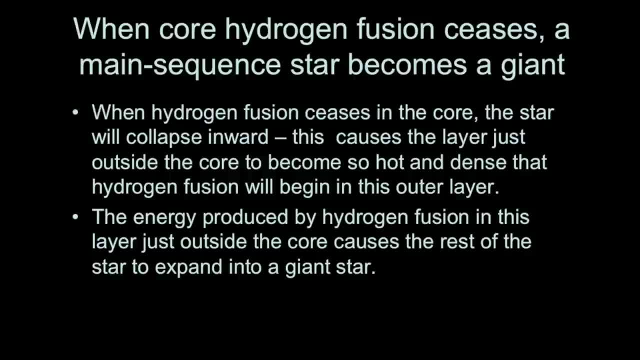 core that they begin fusing, and it's even hotter than the core of the star was before. The hydrogen fusion that begins in this shell is happening at such a fast pace that the outward gas pressure that results from this shell fusion makes the outer layers of the 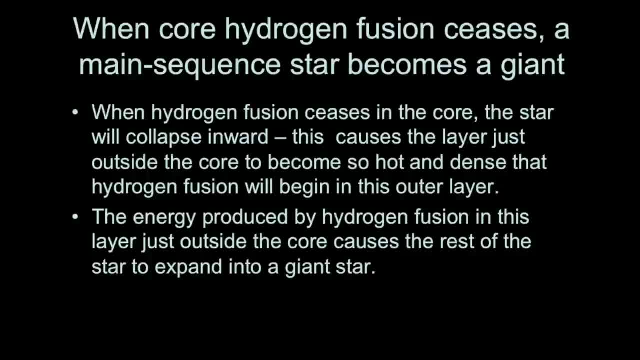 star expand even further than they were when the star was a main sequence star, And so the star will expand and because of this, on the outside, as it gets larger, it will become brighter than it was before And it will also lose zoonosis. 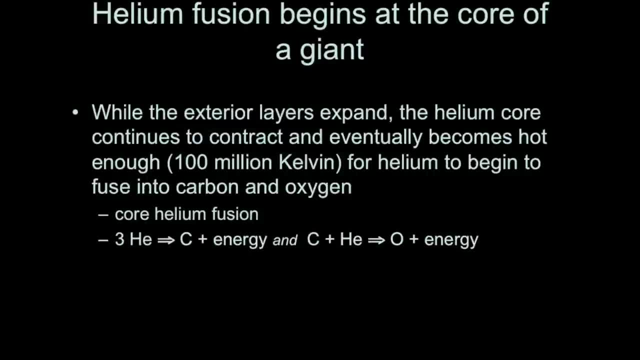 It will lose some surface temperature. Eventually, the core of the star, which is all helium at this point, will collapse down to the point where its temperature is in excess of 100 million Kelvin. At this point the helium atoms can fuse into carbon and oxygen. 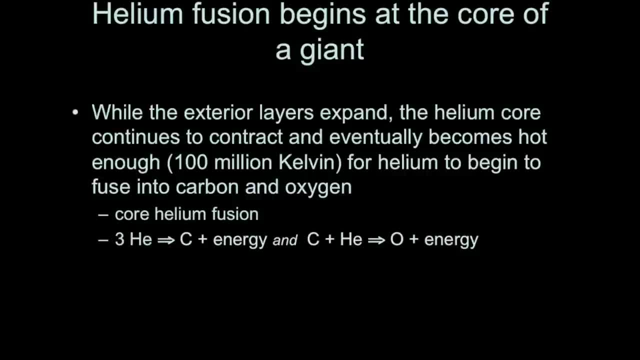 And so you get a new set of nuclear processes. This isn't hydrogen into helium, This is helium into carbon, This is hydrogen, and also helium into oxygen. And so what are the net reactions? You have three heliums can fuse into a carbon. 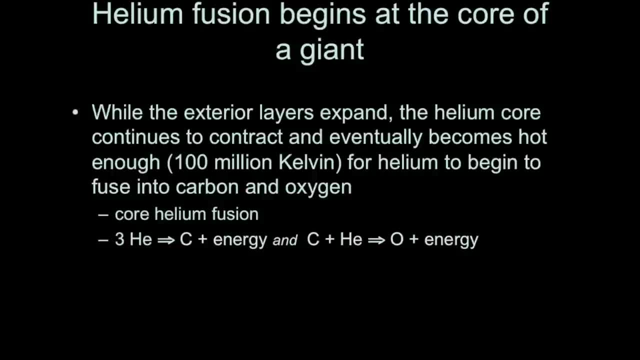 You get some energy out, Or you can also have a carbon plus a helium and build an oxygen And you also get energy out. this way, These reactions are going to happen at a much faster pace than the hydrogen to helium reactions that were occurring during the main sequence lifetime of the star. 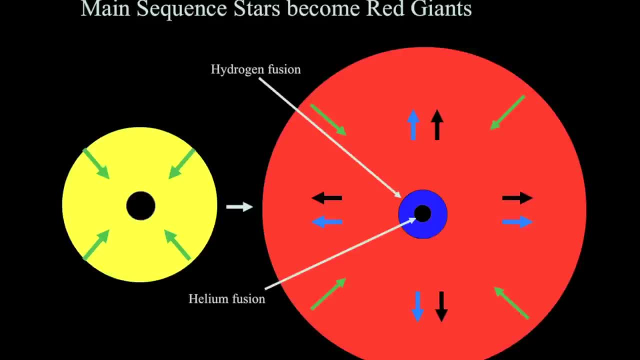 And so later on in the star's life cycle we're going to see a reaction that's going to happen at a much faster pace than the hydrogen to helium reactions that were occurring during the main sequence lifetime of the star. Later on in what we call the red giant lifetime of the star, we've gone from having a star. 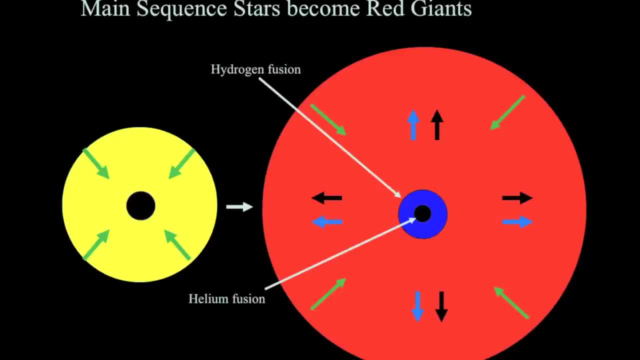 expanding and getting larger, while the core is crushing down and getting smaller. Eventually, the interior of the star will have layers that look like this, where there's a core represented by the black dot in this picture. That's where the helium fusing is taking place, the helium fusion. 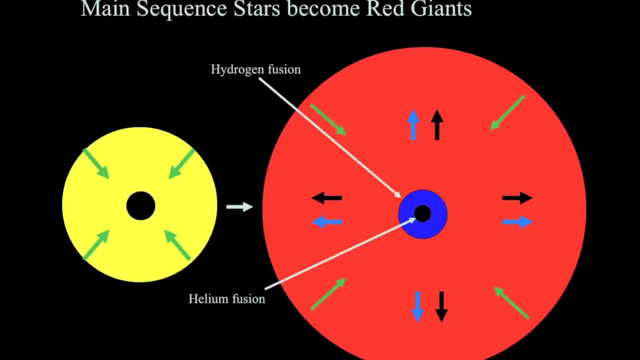 Helium is fusing And a carbon and oxygen nuclei Around the core is a hot, dense shell of hydrogen material, And that material is fusing, generating an outward flow of energy That is sustaining a gas pressure which has pushed the outer layers of the star much farther. 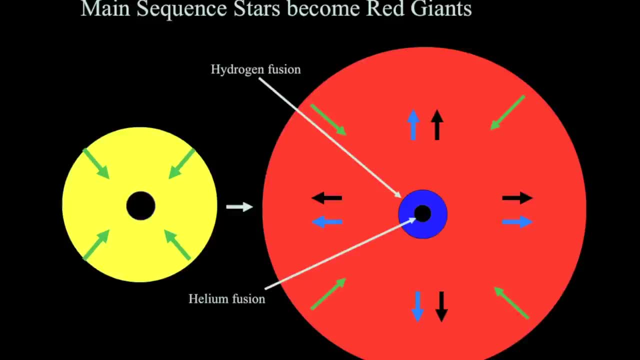 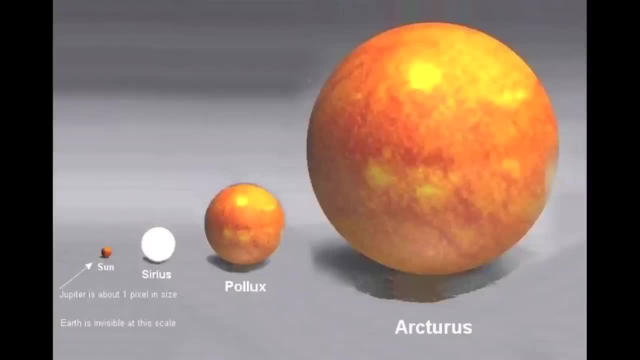 out than they were before And the outer layers are still just hydrogen. and those far outer layers are not fusing into any new elements. When a star has expanded to this point, it's much larger than it was during the main sequence lifetime. 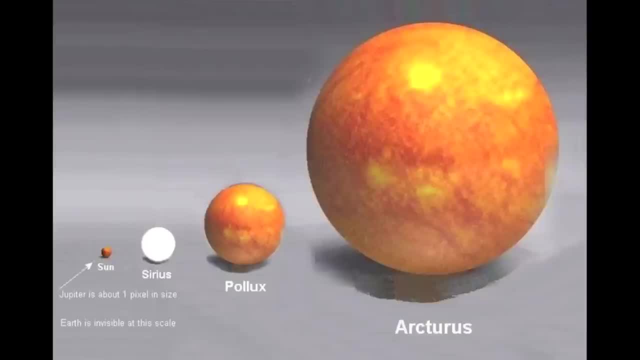 The image that I'm showing you here shows the Sun as a main sequence star, relative in size to a few other stars- Sirius, Pollux and Arcturus. But let's take a look at these stars compared to their red giant analogs. 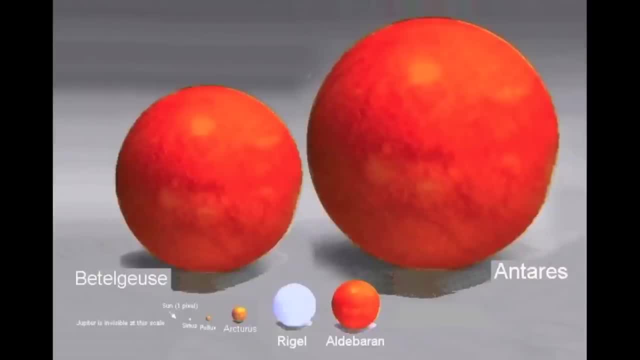 So the Sun in this new image is just one pixel in size. But look at Betelgeuse and Antares. These are red giant stars. These are stars that have expanded after the main sequence lifetime to tremendous sizes. Betelgeuse and Antares are so large that if you were to place them in our solar system, 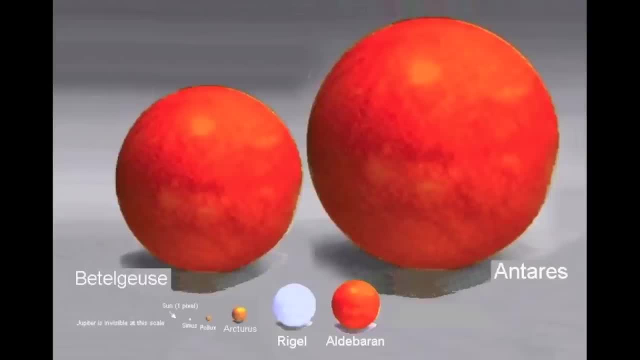 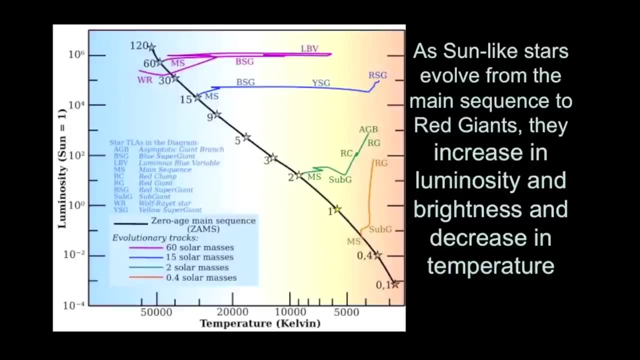 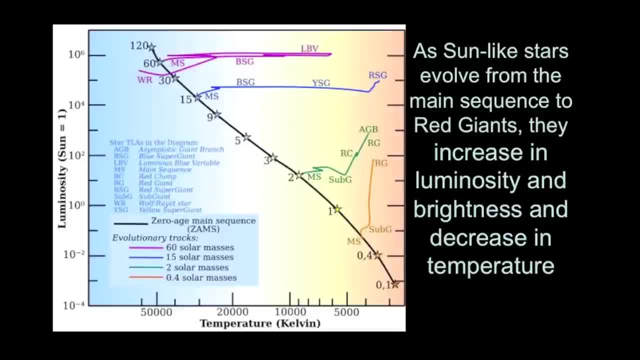 Here is an example. Here is an example. Here is an example on the HR diagram. We have a main sequence that is depicted in this HR diagram represented by the bold diagonal line, and along this line are star symbols that represent main sequence, stars of different masses. 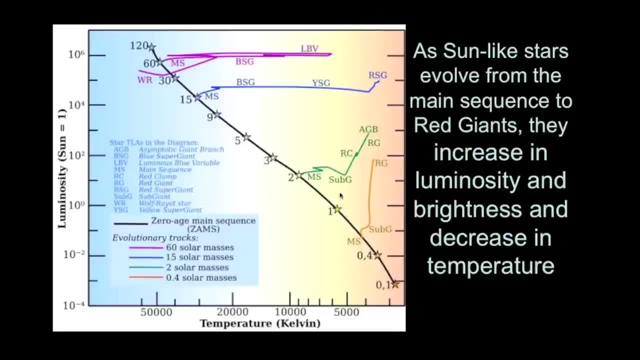 and so our Sun would have a main sequence mass of one solar mass. here's a star of two solar masses, 5, 9, 30, and so on. The other lines, the other colored lines that are represented here on this HR diagram, are the property tracks. 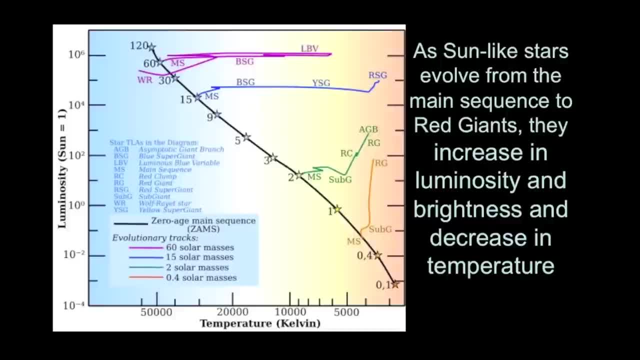 of stars of different masses after they finish their main sequence lifetime. so for a star that is about half the mass of the Sun- I'll point to it here- it's labeled as MS. this star will expand after its main sequence lifetime and as it becomes larger it'll become brighter and it will also decrease. 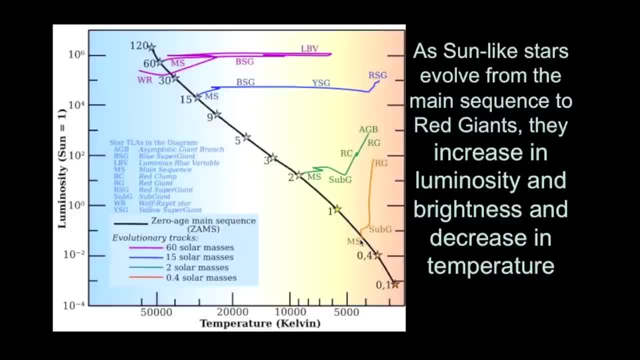 very slightly in surface temperature, and so, as we follow its life track into the main, after the main sequence, into the red giant branch, it will go up in luminosity, and that's because it's becoming brighter- a star that is two times the mass of the Sun. 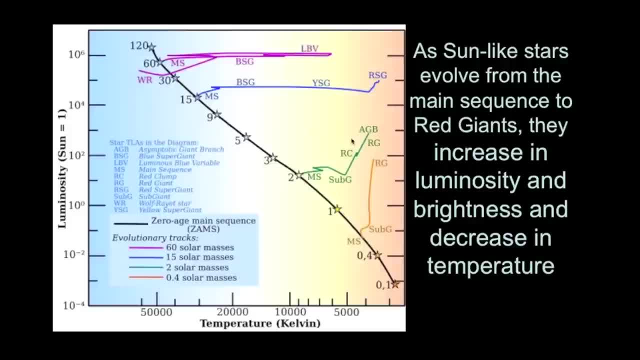 so not much more massive than the Sun, will begin as a main sequence star on this on the bold line, and it will go to the right, decreasing in surface temperature, but eventually will increase in luminosity. what happens here is that this star will eventually expand to the point. 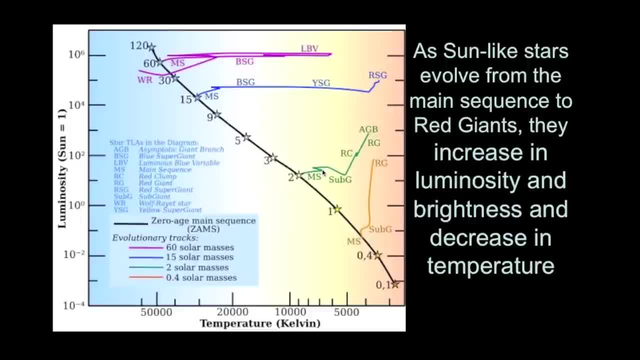 where its decrease in surface temperature on the outer layers are, are different from what's happening in the core. the core will eventually begin fusing helium into carbon and oxygen, and when that happens, the core will eventually begin fusing helium into carbon and oxygen when that occurs. 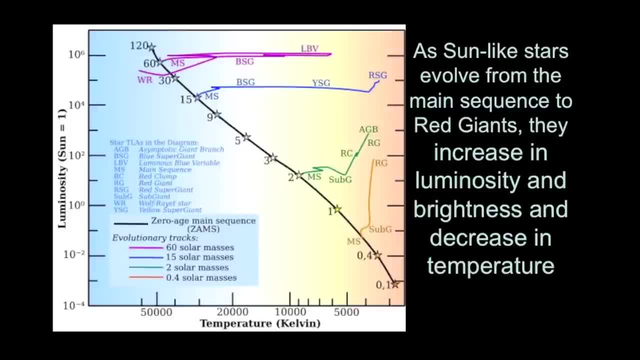 the star will truly be a red giant. more massive stars have different life tracks. they can go beyond the fusion of helium into carbon and oxygen, and they can fuse even heavier elements, but we'll talk about that in another video. however, their life tracks take them from extreme luminosities. 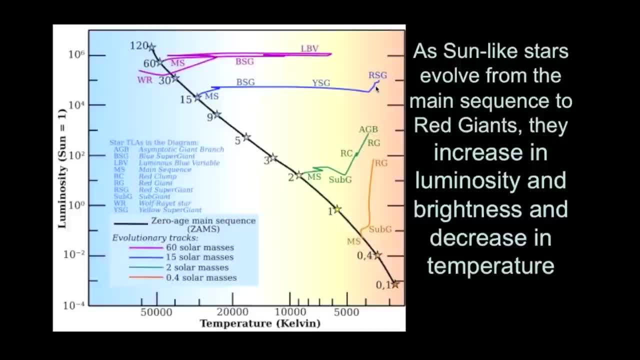 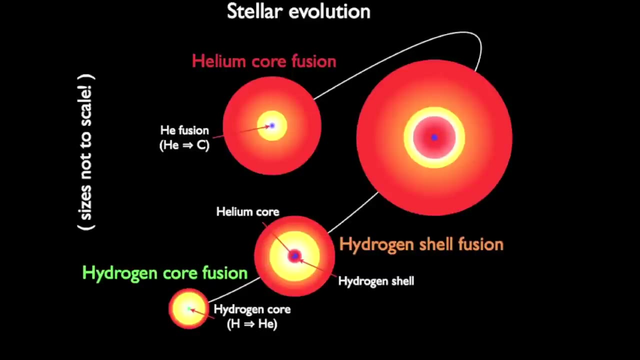 to similar luminosities but very low surface temperatures, and so I've circled here the life track which is most similar in this image to the life track of a Sun-like star. here's another schematic of the different layers that you would have in these different 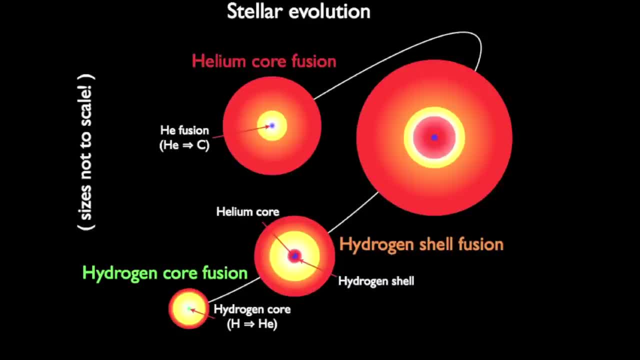 times during a after the main sequence lifetime of a star. so during the main sequence lifetime of a star, you would have hydrogen fusion in the core, that's hydrogen into helium, and then you'd have a helium core. after the main sequence lifetime there would be a hydrogen shell that develops. 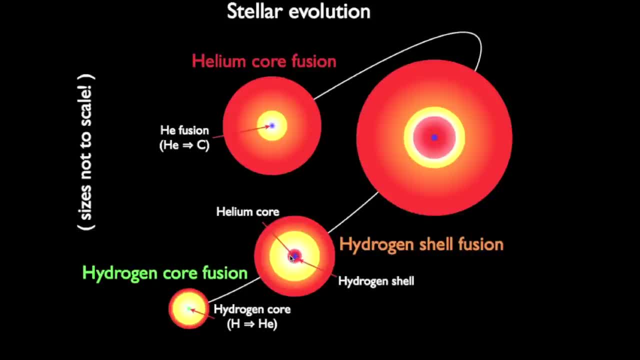 around that and that causes the outer layers to expand to a larger size. eventually, that shell fusion causes the star to expand to such a large size that it's extremely high in luminosity. however, when a star begins helium core fusion, the outer layers will contract down very slightly. 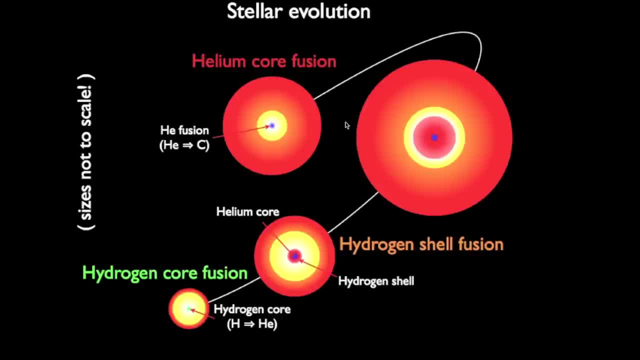 and so the red giant star, when it finally becomes a helium fusing red giant, is just slightly smaller than before, and so it'll lose a little luminosity. but a red giant is a red giant when it is fusing a helium into carbon and oxygen in its core. 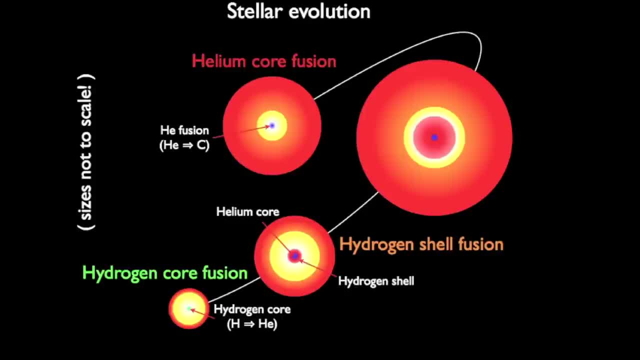 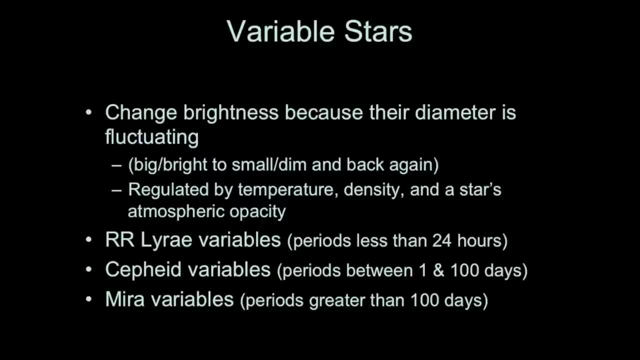 and so this sort of fusionifiebs helium to oxygen in it's core, And so this is the life of a star after it has finished its main sequence- lifetime. Also, another thing can occur When a star becomes a red giant. during this process, it's expanding out. 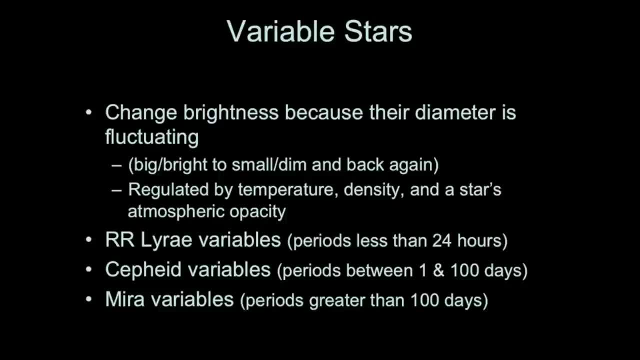 but gravity may pull some of the layers back inward And when that occurs, some of these inner layers will get hot and denser and will cause an increase in the energy generation on the inside of the star. This will cause the outer layers to want to expand again and gravity may pull back. 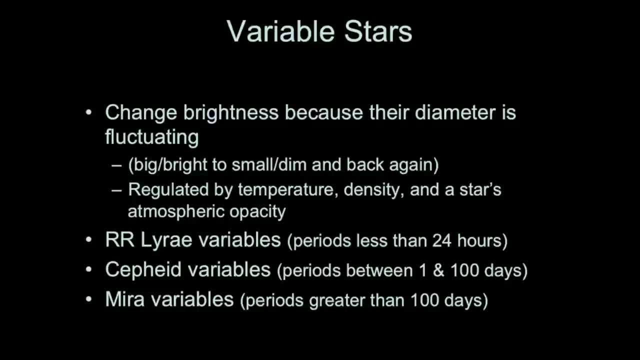 This oscillation between gas pressure and gravity can cause a star, a red, giant star, to be what we call a variable star, And so it will get larger, it will get smaller, and that will result in it appearing brighter and dimmer over time.